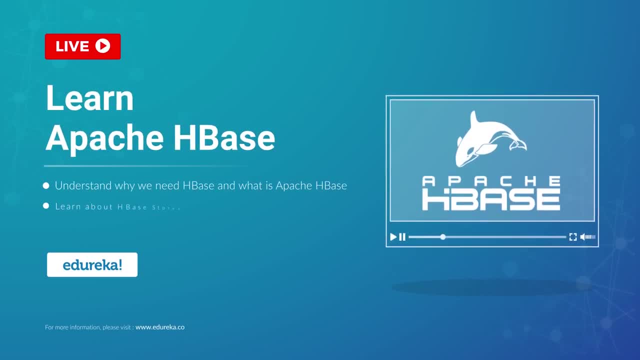 So good morning, good afternoon and good evening, guys, based on the time zones you all are coming from. So, guys, before we start with the session, can you all please give me a quick information, if you all can see my screen and hear me loud and clear as well. 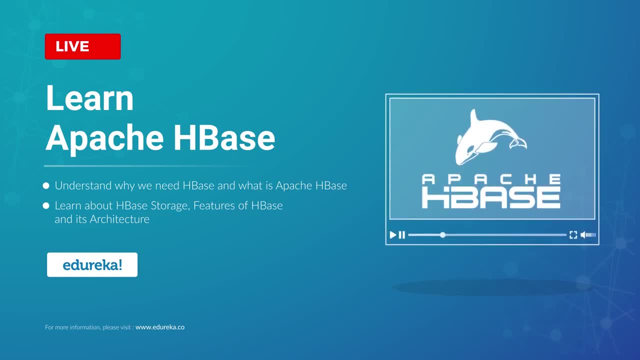 Perfect. Thank you for the confirmation, everyone. So before we get started, let me quickly introduce myself to you all first. So my name is Neeraj Khadia and I have been working in this IT industry for more than 13 years now. So today we have gathered for a discussion mainly on 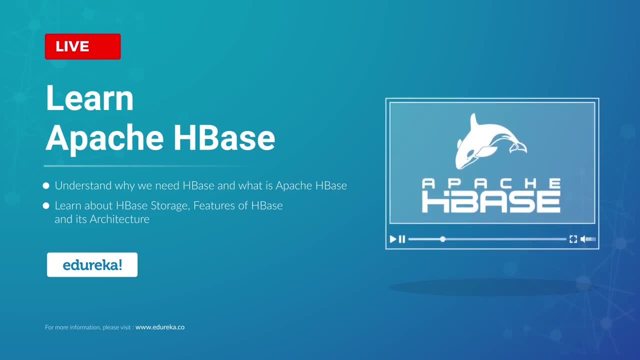 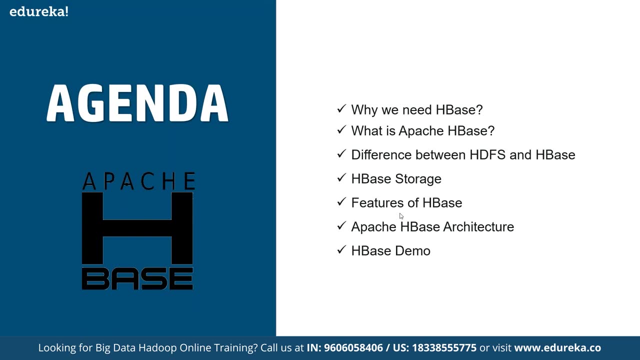 how the Apache Edgebase is structured. So today we are going to discuss on why exactly we need Edgebase, what exactly that is the main use of using Edgebase here, How the concepts of HDFS and MapReduce are structured and how we can use Edgebase as. 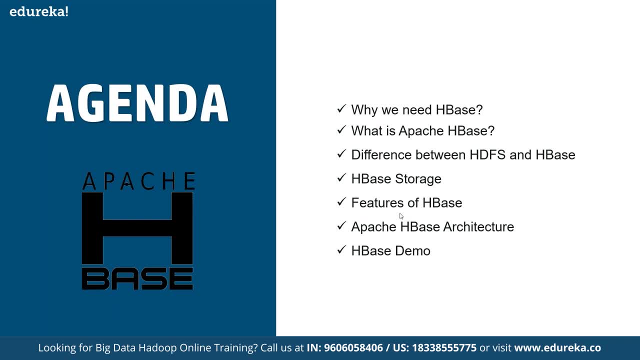 a part of our big data analysis And then, if the time allows, and we also going to see a quick hands-on on the Edgebase topic that we're going to discuss here, All right, so let's get started. So if we talk about why exactly we need Edgebase, then data we know will be accessed only in 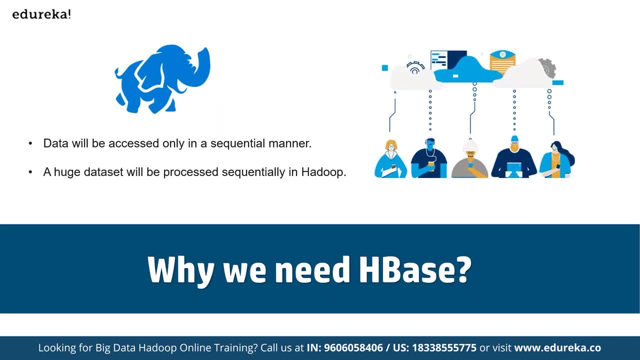 a series Equation manner. So, for example, when we are running a big data analytical job here, then for that we know that data is going to be run in an in a given sequence, And that's why we can use the HD base storage structure instead of using the random access. 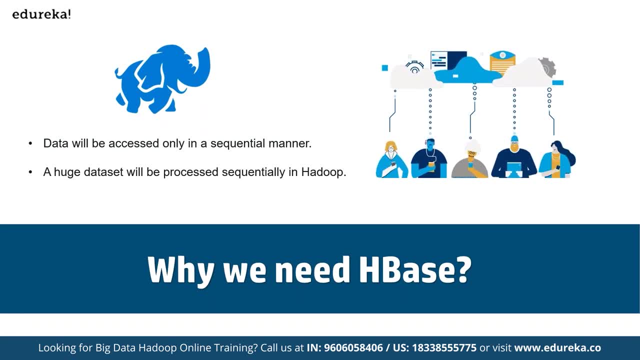 optimized SSDs. So if you talk about the Edgebase first, again, Edgebase is what Edgebase is basically a part of the Hadoop ecosystem and where we can make use of Edgebase in order to make sure we are having an effective data. 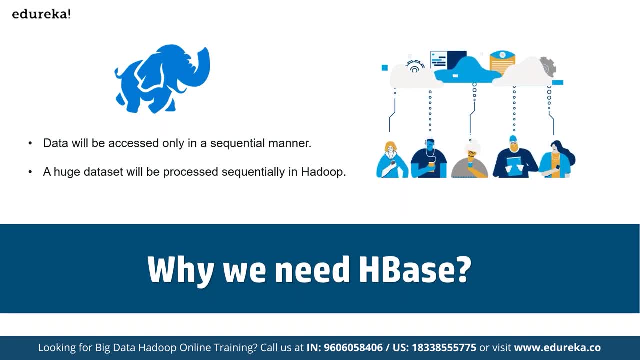 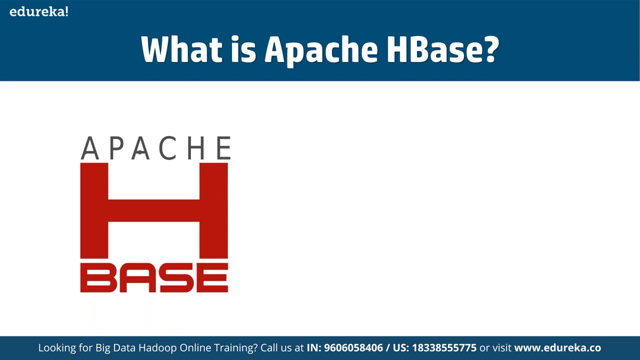 Structure in that to in different nodes and then how we can fetch that for completing our big data analysis. Any huge data set will be processed sequentially in Hadoop, especially for the large volume of data sets. Correct, Now, if we talk about a bit of small history here, then Edgebase is modeled after Google's. 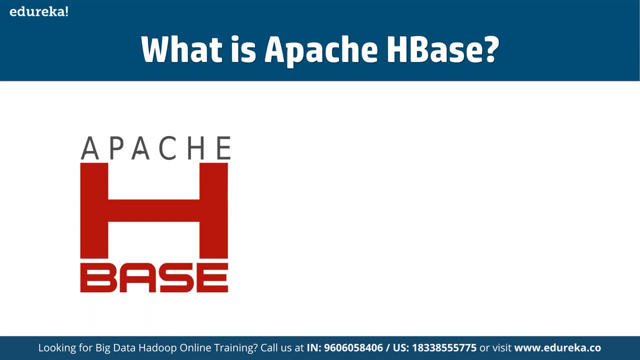 big table which is used to collect data and serve requests for various Google services like Maps, Finance, Earth, etc. And Apache Edgebase began as a project By the company power set for natural language search, which was handling massive and sparse data sets, and Apache Edgebase was first released in February 2007.. 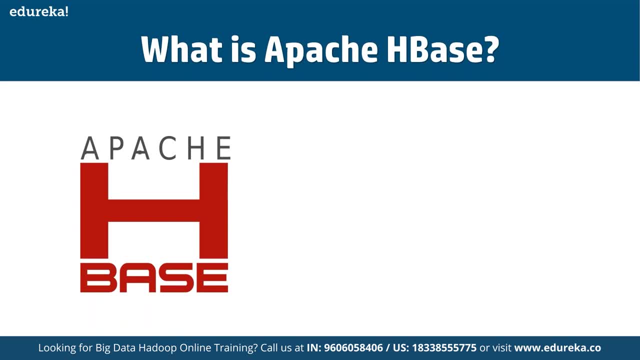 And later, in January 2008,, Edgebase became a sub project of Apache Hadoop. Now, in 2010,, Edgebase became Apache's top-level project. So if you talk about the Edgebase tutorial, then Edgebase is an open-source, multi-dimensional. 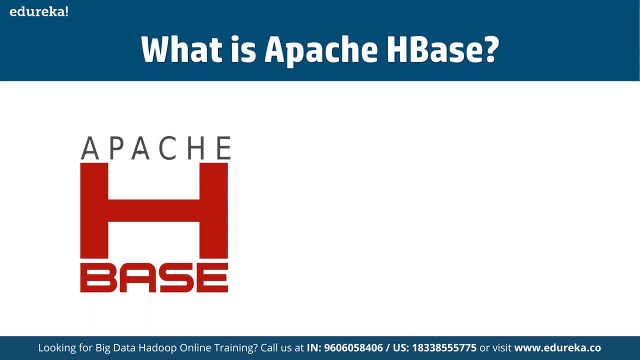 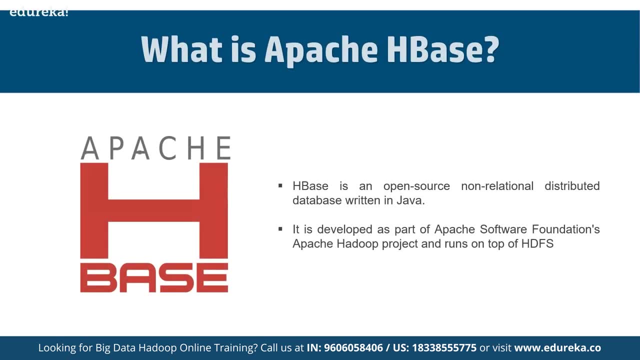 distributed, scalable and no SQL database within it. So Edgebase, as we discussed. Edgebase basically runs on top of HDFS, as in Hadoop distributed file system, and it provides big table like capabilities for to Hadoop. Now it is designed to provide a fault-tolerant way of storing large collection of sparse. 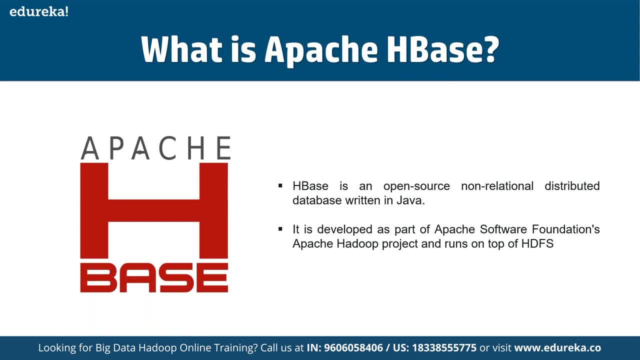 data sets. Now, since Edgebase achieves high throughput and low latency by providing faster read write access on huge data sets, It is Used for the applications where we need to have a fast and random access to large sets of data. So, basically, compression in memory operations and bloom filters that we have for data structures. 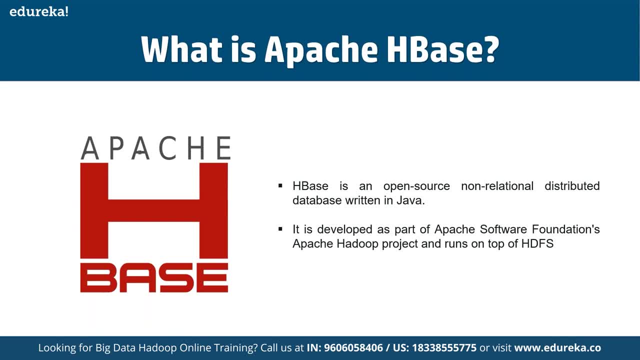 which tells you whether a value is present in a set or not. So these features are available here to fulfill the requirement of fast and random read write operations. Now we can understand this by a simple example. Let's say a jet engine generates various types of data. 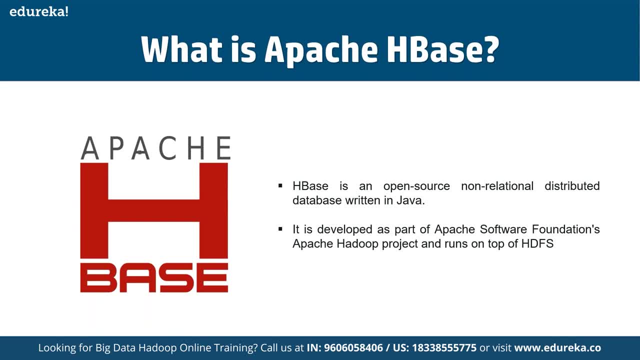 From different sensors, like pressure sensor, temperature sensor, speed sensors, Etc. which indicates the health of the engine. Now. this is very useful to understand the problems and status of the flight. Now, continuous engine operations generates 500 GB of data per flight and they are 300,000. 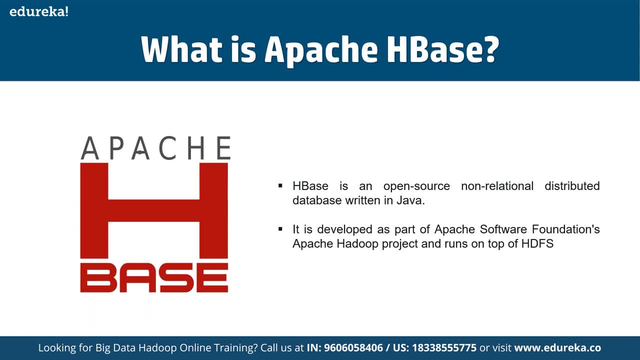 flights per day approximately Right. So engine analytics applied to such data in near real time can be used to proactively diagnose problems And reduce unplanned downtime, and this requires a distributed environment of handling large data volume with fast random read and write for real time processing, and here edgebase. 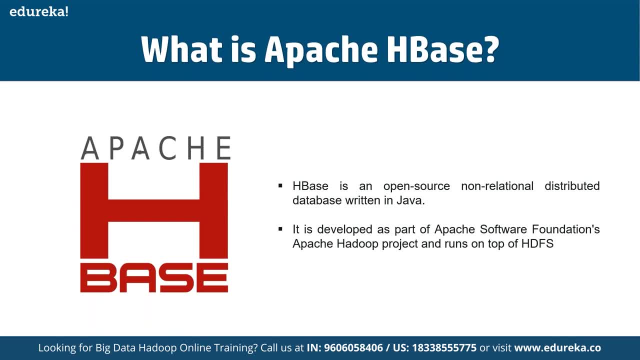 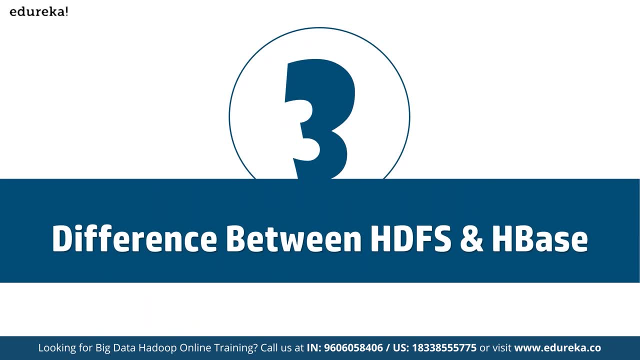 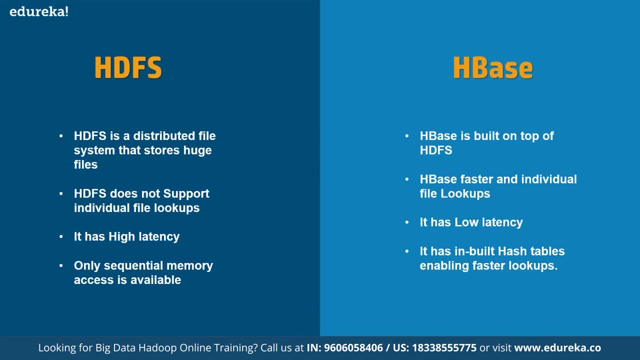 comes to the rescue. So we are going to talk about edgebase again as you proceed further. Now, if you talk about the main difference between HDFS and edgebase, then we know that HDFS is what HDFS is Basically: a Java based distributed file system that allows us to store large data across multiple 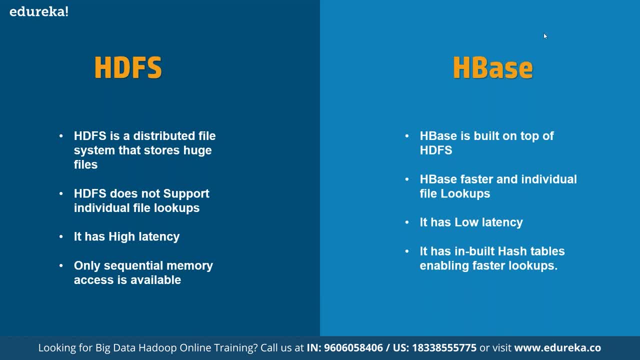 nodes in a Hadoop cluster. It has its own well-defined architecture put in place. So, as you can say it's it's basically an underlying sewing system for storing data in the distributed environment, and HDFS is basically a file system, Whereas edgebase is a database itself. 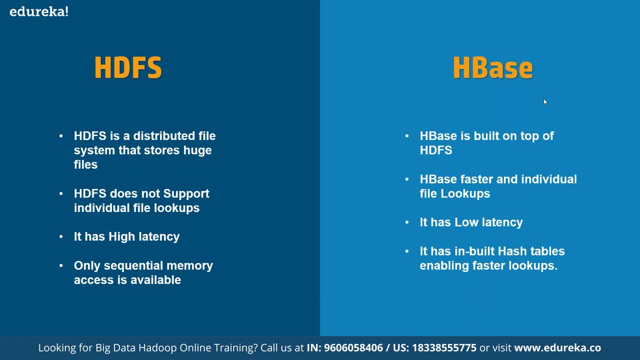 Similar to entry, Similar to mysql Now, as both HDFS and edgebase stores any kind of data that is structured, semi-structured and unstructured in a distributed environment. So let's look at the differences between HDFS and edgebase. So we know, have seen again, as we can see here, edgebase provides low latency access to small amounts of data. 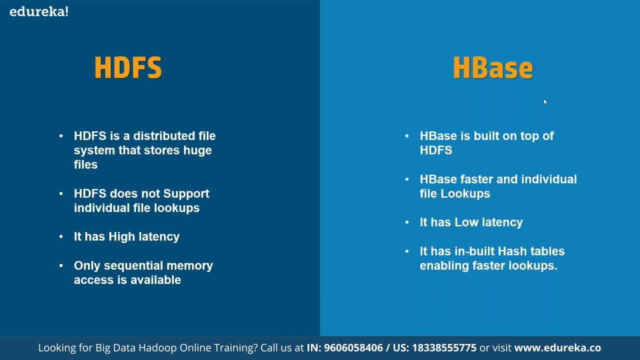 within large data sets, while HDFS provides high latency operations and edgebase supports Random read and write, while HDFS supports worm worm, as in write once and read many or multiple times, And HDFS is basically- or we can say primarily- access through MapReduce jobs, while edgebase is access. 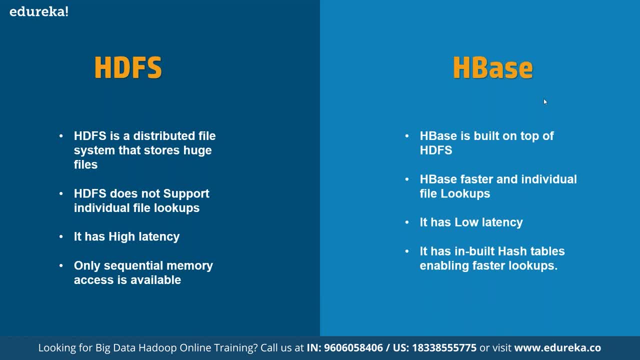 through shell commands, Java APIs, rest, Avro or thrift APIs and HDFS stores large data sets in distributed environment and leverages batch processing on the data. For example, it would be Helping and any e-commerce store to store millions of customers data in a distributed environment. 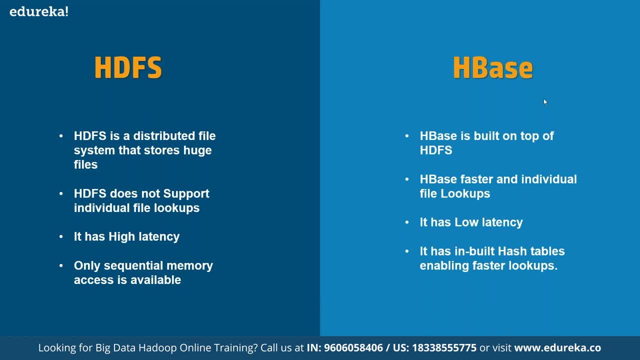 which grew over a period of time. For example, maybe it may be four or five or six years old. Then it is going to leverage batch processing over data and analyze customer behaviors, patterns and requirements. So then the company could find out what type of product customer purchase in which month, and it simply helps to store. 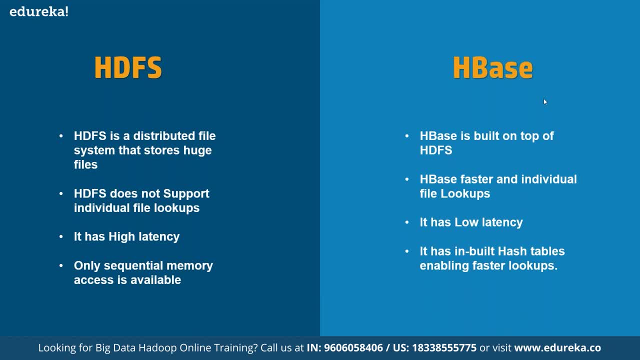 archive data and execute batch processing over it. So, while the edgebase stores data in a column oriented manner, which where each column is stored together so that reading becomes faster and leveraging the real-time processing, For example, in a similar e-commerce environment, it stores millions of product data. 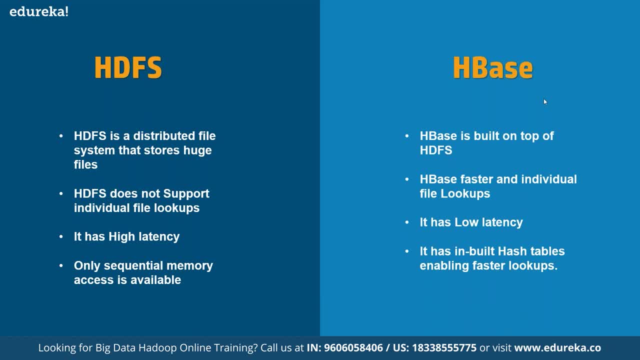 So if we search for a product among millions of products, it optimizes the request and search processes, So producing the result immediately, Or we can say In real time set up. So the deep now again, and the exactly is what we are going to discuss when we start our session, all together on top of big data. 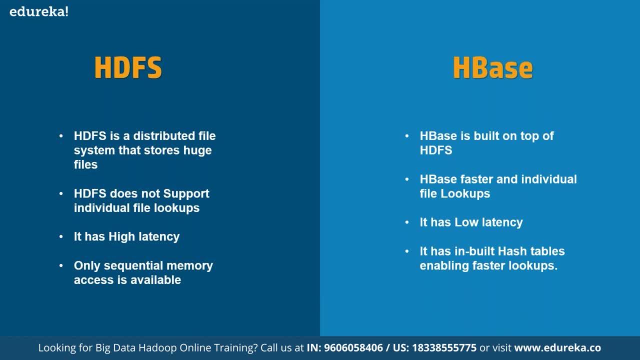 where edgebase is a fully focused module. Now, as we know, edgebase is basically are distributed over HDFS. So combination of both can give us great opportunity to use the benefits of both and tailor situation. We can use the begin for samples here here. 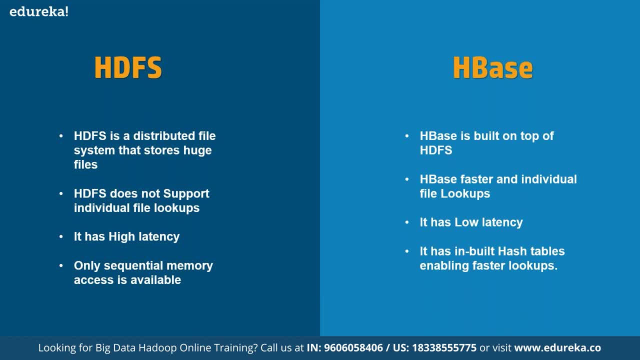 We can also take a sample For Facebook passenger case study as well, in case you want to understand it further. So, if you talk about Facebook now, Facebook messaging platform shifted from Apache Cassandra to edgebase in November 2010.. So, again, that is not the part of the content here. 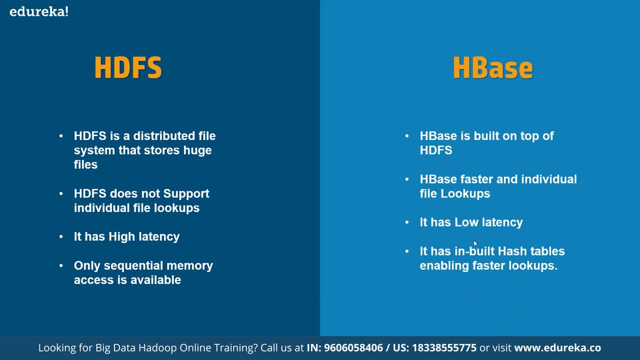 But anyways, I'm going to give you a small overview for that. So Facebook messaging platform was transferred was transferred to edgebase back in November 2010.. So Facebook messenger combines messages, emails, Chats and SMS in a real-time conversation. So Facebook was trying to build a scalable and Robo's infrastructure to handle a set of these services. 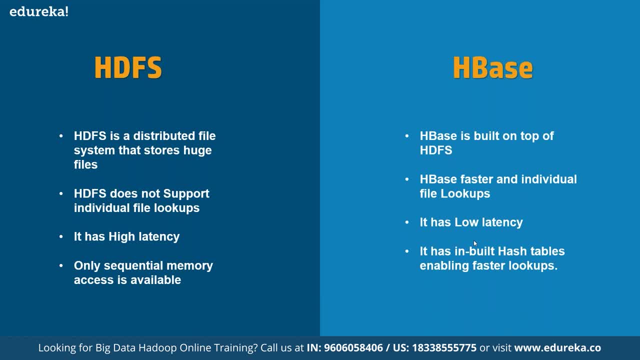 Now, at that time, the message infrastructure handle over around 350 million users sending over 15 billion person-to-person messages per month. That was a human. this amount of data and the chat service supports over 300 million users who send over 120 billion messages. 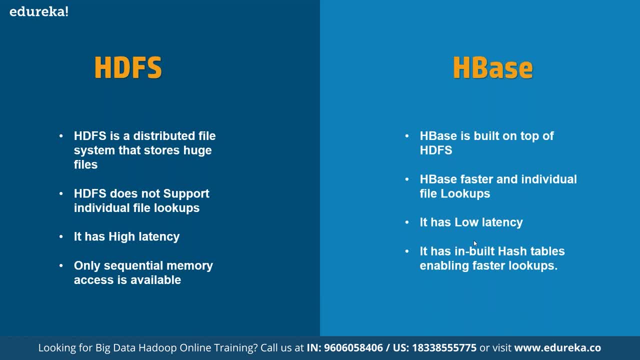 So that was a human. this amount of data and the chat service supports over 300 million users who send over 300 million messages per month basis. So, by monitoring the usage, they found out that two general data patterns were observed. So a short set of temporal data that tends to be volatile and an ever-growing set of data that really gets access. 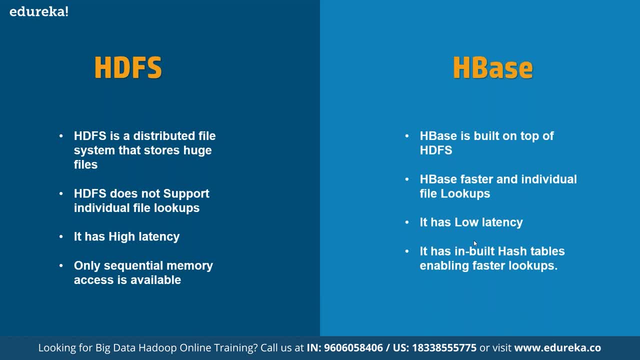 So Facebook wanted to find a storage solution for these two usage patterns and they started investigating to find a replacement for the existing messaging infrastructure. So earlier In 2008 they use open-source database, like we have Cassandra, where it is basically an eventual consistency key value store that was already in production serving traffic for inbox search. their teams had a great knowledge in using and managing a mysql database. 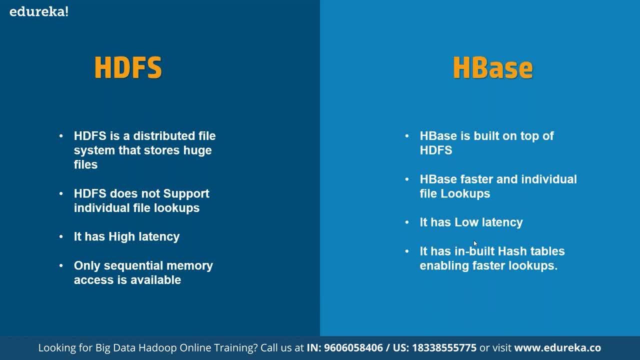 So switching either of the technologies was a serious concern for them and they spend a few weeks testing different frameworks to evaluate the clusters of mysql, Apache, Well, Apache, Cassandra, Apache, HBase and other systems and the ultimate selection. I was done for HBase now, as mysql failed to handle large data set efficiently. as indexes and data set grew large, the performance suffered. 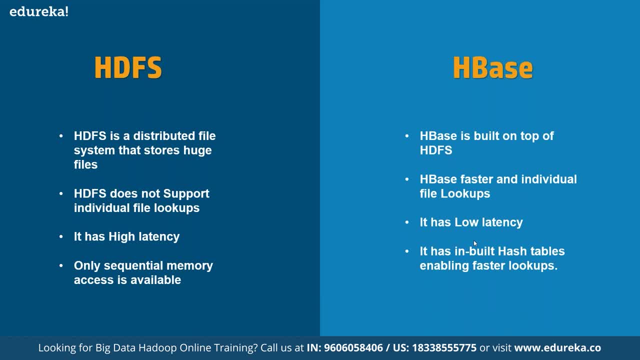 and they found Cassandra unable to handle difficult pattern to reconcile their new messages infrastructure, All right. So basically they were multiple problems face here and that was resolved All all by using edgebase that we are going to discuss as we proceed further. so if we talk about the 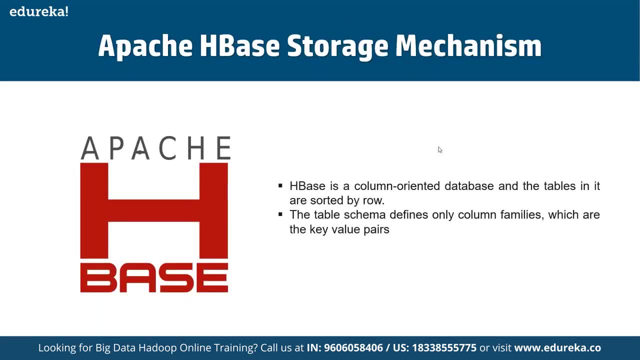 edgebase storage mechanism, then edgebase is what? edgebase is basically a column oriented database. so the table schema defines only column families and key value pairs. so that's why we can see: edgebase is what edgebase is what- a simple no sql database. so it's not an sql database, it's not. 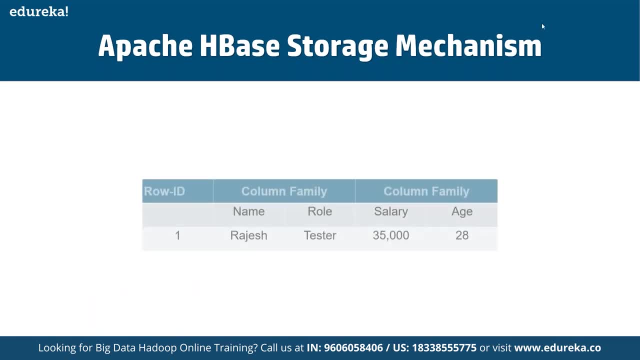 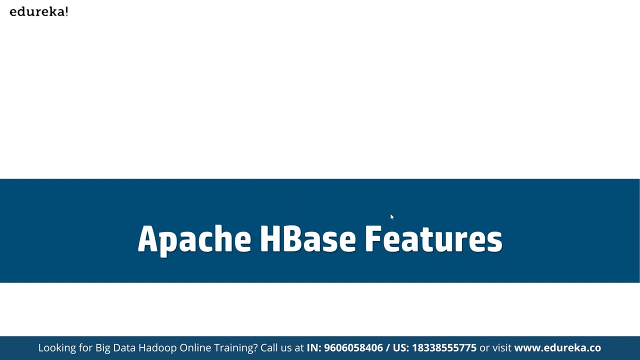 a part of the relational database service, but it's more like a complete no sql database service, like we had dynamo db, we have cassandra, so these are what no sql database is. so, for example, here we have to find a row id, row id, and then we have column family as name and role. now, here, if you, 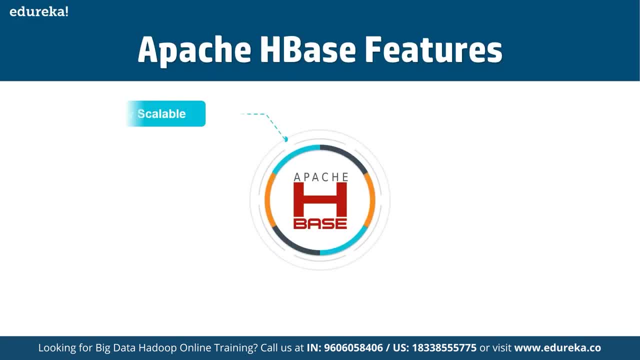 talk about the edgebase primary features, then edgebase, first of all, can be scaled linearly. that means again, we can increase the capacity, we can increase this number of rows that we can store here at any point of time. then it also supports auto failure support by maintaining a standby structure. 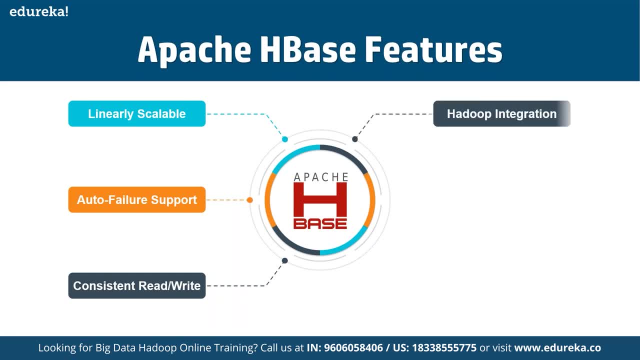 it offers consistent read and write, and we also have the inconsistent reader nights up for support also available. then we have- and again it can be easily integrated with hadoop, because again it is one primary tool being used here, and again it offers a good java api support as well. 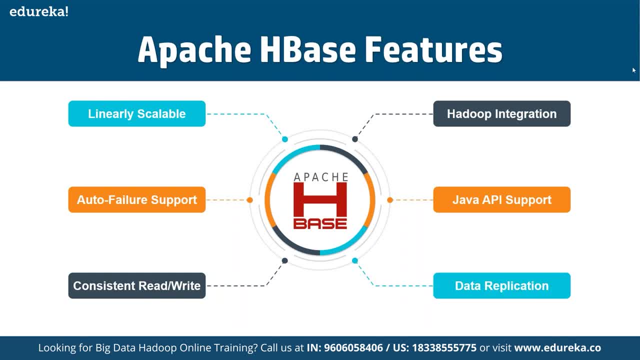 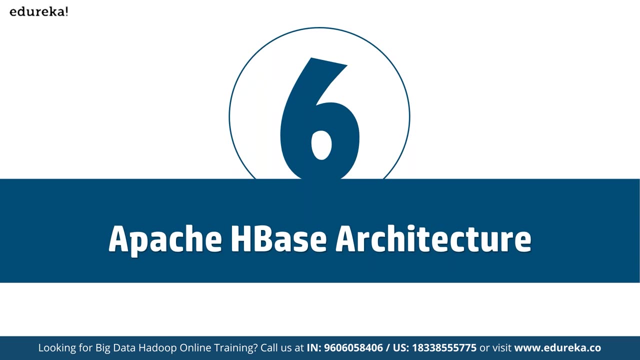 and now and then, if we are using edgebase and to increase the resiliency of the architecture, we can simply replicate data from one part to the other. now, if we talk about, let's talk about the apache base architecture. so, as we know, edgebase is what? edgebase is basically a column oriented, no sql. 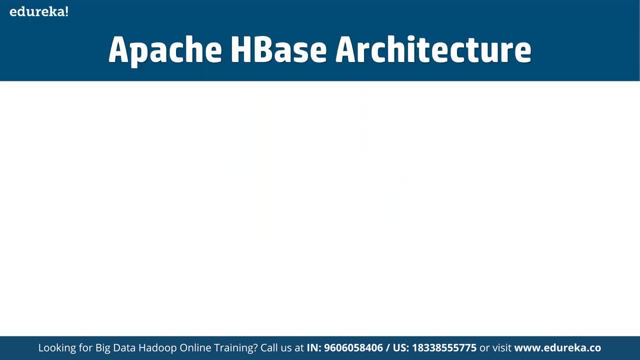 database now, although it looks similar to a relation database, which contains rows and columns, but it is not a relational database, right? so relational databases are now are row oriented, while edgebase is a column oriented structure. so let's understand the difference between column oriented and row oriented databases. so if we talk about row oriented versus column oriented database, 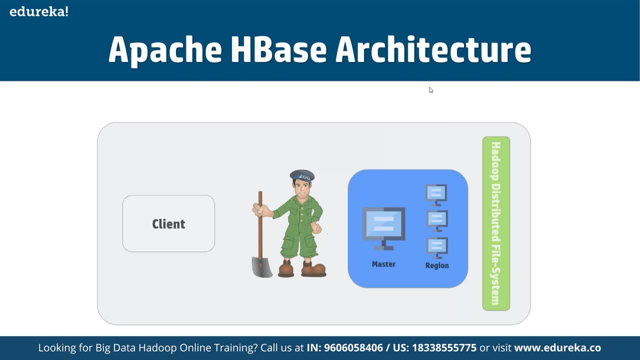 then, row oriented databases store table records in a sequence of rows, whereas column oriented databases store table records in a sequence of columns, that is, the entries in a column are stored in contain in it's in a continuous location on disk. all right, so it's basically here. we can assign regions to the region servers and take the help. 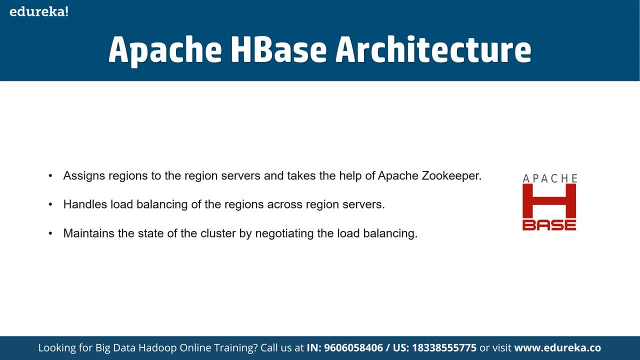 of apache zookeeper. so basically we are also going to handle load balancing of regions across region servers and then we can maintain the state of the cluster by negotiating the load balancing itself, and then it allows a good communication with the client and handle data related operations and how. 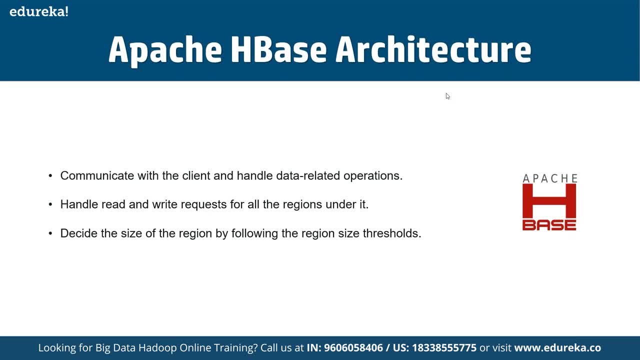 it also allows us to handle, read and write requests for all the regions under it, and then it decides size of the region by following the region size as available here. so if you talk about region, then a region contains all the rows between the start key and the end key assigned to that region. so 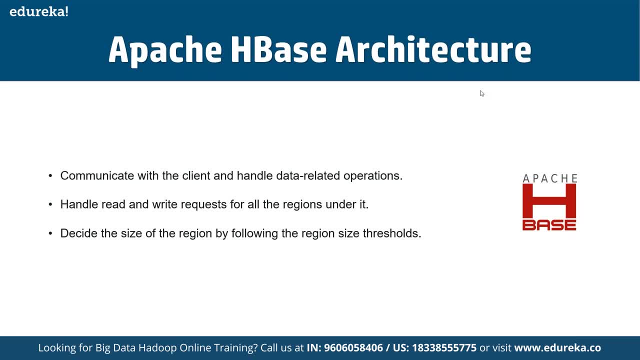 edgebase tables can be divided into a number of regions and in such a way that all the columns of a column family is stored in one region, so each region contains rows in a sorted order. so many regions are assigned to a region server, which is a responsible for handling, managing and executing reads and write operations on that set of regions. 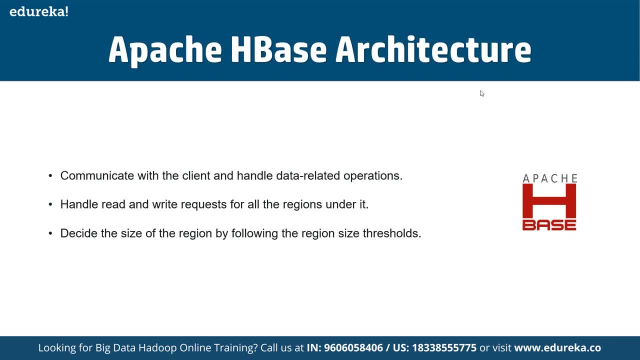 so we can say we can. to summarize, we can say: a table can be divided into a number of regions and a region is basically a sorted range of rows storing data between between a start key and the end key, and a region has a default size or 256 mb, which can be configured according to the need. 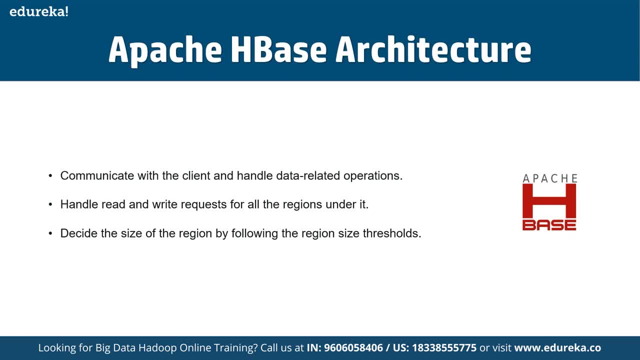 and a group of regions is served to the client by a region server, and a region server can approximately serve a thousand regions to the client here now, starting from the top of the hierarchy, we can explain. we can again. we can explain in detail about the edge master server, which acts similarly as a name node in hgfs. 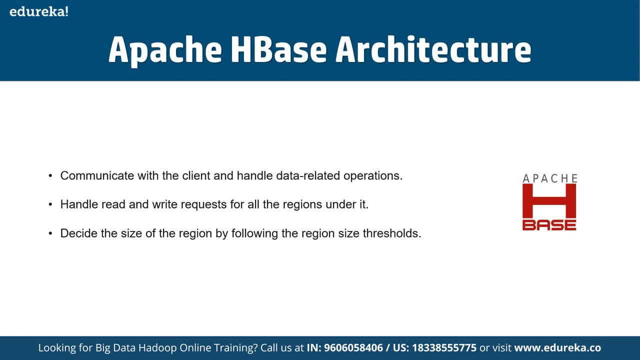 and then, moving down in the hierarchy, we are going to talk about the zookeeper and region server as well. so as a part of the architecture, we also have edge master as well. so edge master is also used for handling a connection of region server which resides on a given data node. 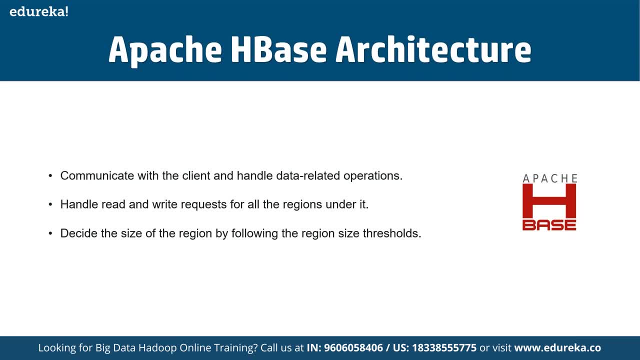 so we can say edge master master. edge base master provides ddl as in data operation and operations to create and delete tables, and it also assigns regions to region servers, as we can see in the previous title that we have taken a look at, and then it coordinates and manages the region server. 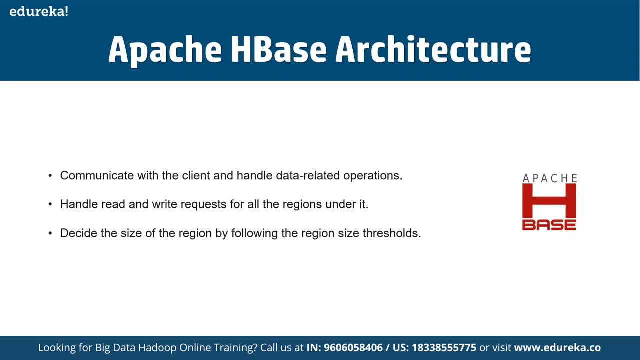 similar to a name node managing data node in hgfs and then assign specific it. it assigns regions to the region servers on startup and reassigns regions to region servers during the recovery and load balancing. and then it monitors all the region servers instantly and that will focus on the clusters from. 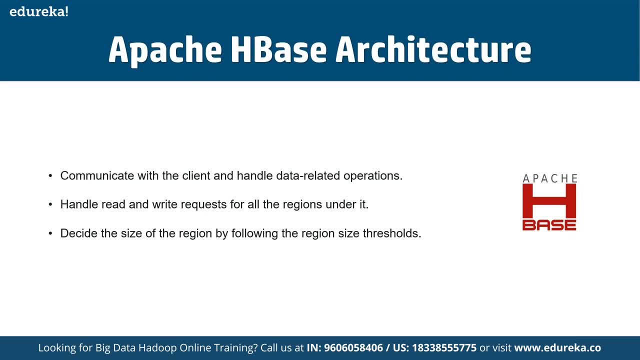 the help of zookeeper itself, and it performs recovery activities whenever any region is down and provides an interface for creating, deleting, parsing table sets as and when required. all right, so now it's a part of a hands-on. we are going to see in how exactly edge base is. 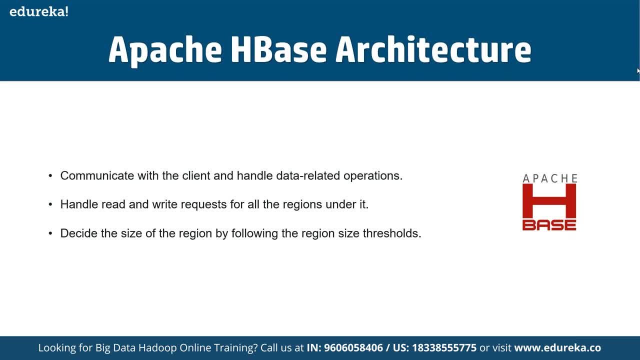 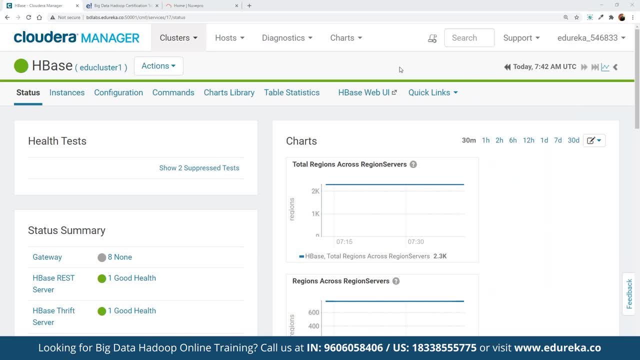 structured. so for that we are going to make use of the cloud leader manager. here we can get the access for getting the access edge base as accordingly we can say available in the cloud manager as well, in case we do have the access to edge based and again, in case we don't have first of. 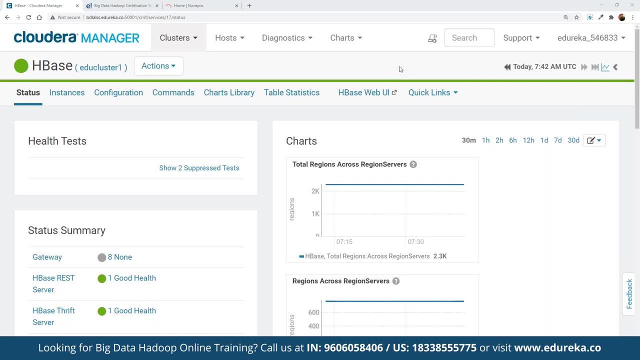 all, we can get the access of some other devices, which we actually like to call coverage, with our edge-based application access to cloud reader live, and we'll be able to work on the edge base package as well once we have installed it. so hue is something that we don't know. is you specifically use as a complete set? 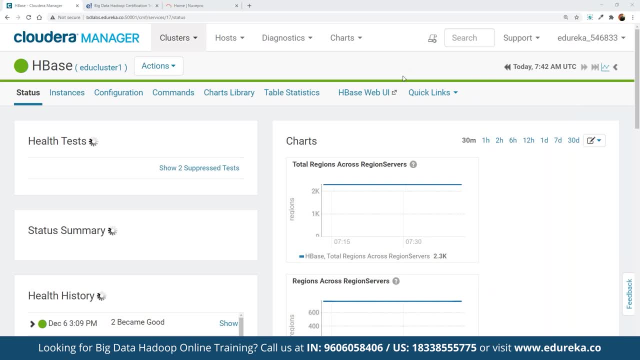 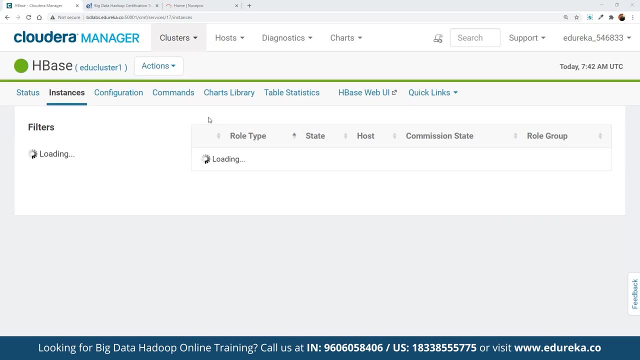 we can say complete file manager itself, and here we can see edge base where we can see the entire base statistics. for example, if in case we have multiple instances up and running for each, we can see the list of all the instances here from the gy where we can see what is the role type. 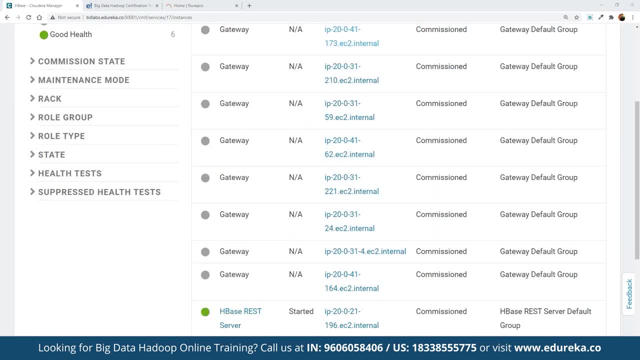 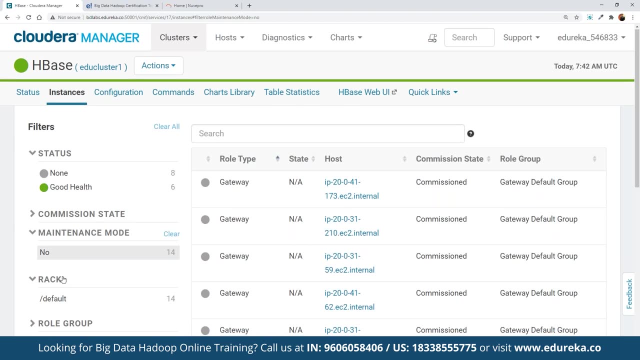 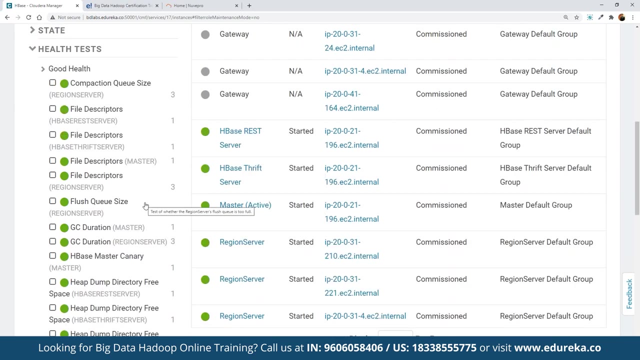 the host, where exactly they are located. here, with the commission state and the rule group available, we can see the entire maintenance mode, which one are in maintenance mode, which one again are currently up and running as default and what exactly the other health tests being conducted and how many instances are currently in file descriptors in compassion queue size. as for the 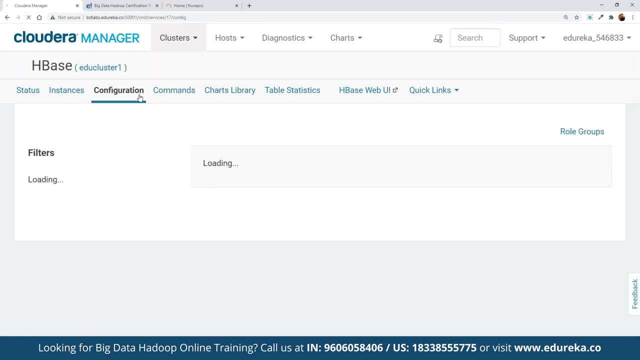 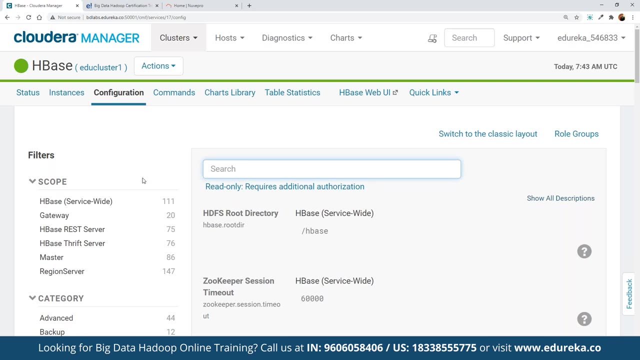 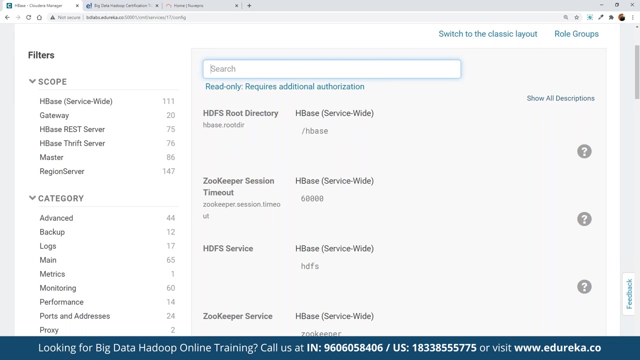 deal report. same way, here we can find the configurations for these instances as a part of the edge based cluster. so we can now- here we can see currently we have how many gateways, edge based stress servers, the gallery in terms of advanced logs, metrics, monitoring and, if you want to use zookeeper for 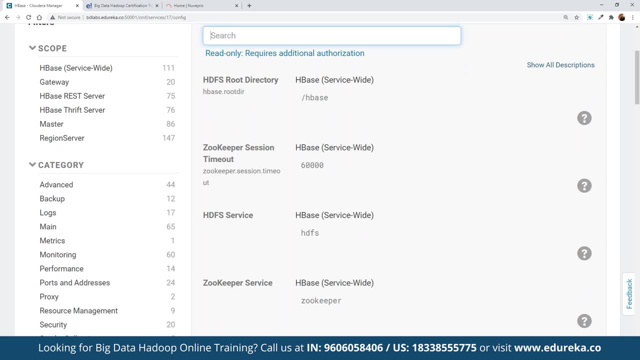 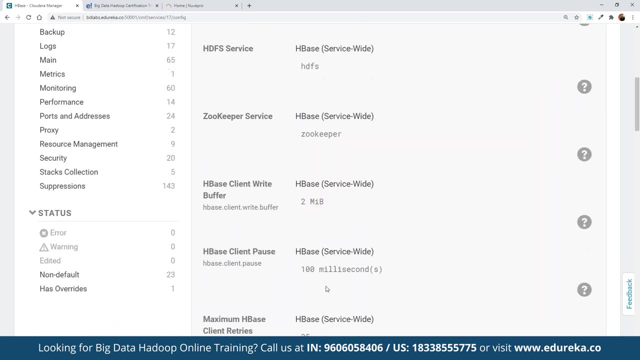 monitoring the service here, then here we can define the threshold as well, which, how quickly we want to monitor it. and then we can define the zookeeper service, the edge based client, right edge based client, what, uh? client pause. so here we can find the right buffer, here we can define: 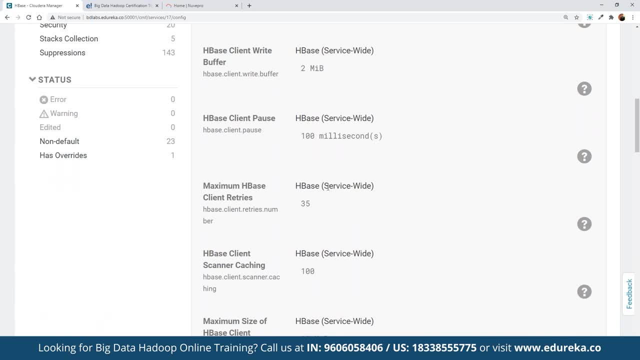 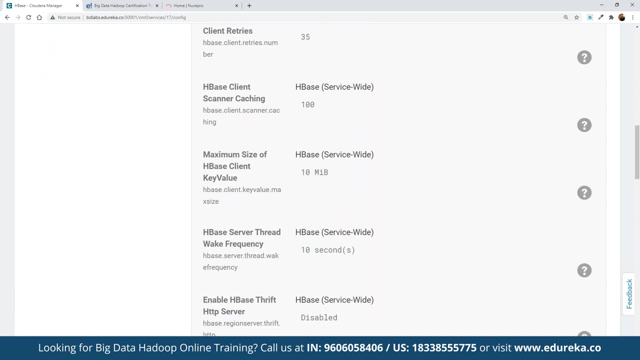 the client pause: here we can define the client address number. the scanner caching: here we can define the key value maximum, the maximum size of the key value we get to find the frequency for the walkthrough. we can say the wave frequency, we can define it for the script. 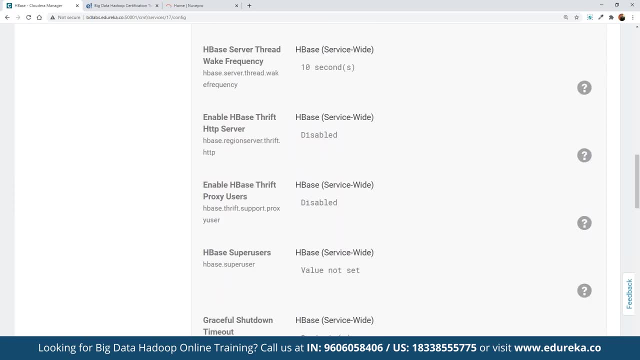 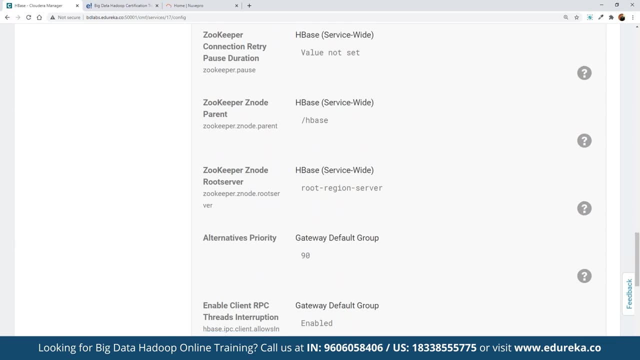 and the proxy user. and here we can find the super users: rpc, diamond, so keep our connection retires. and then the xenode root server. so again that means here we can see the entire configuration defined, for the nodes are going to be available in the configuration tab. 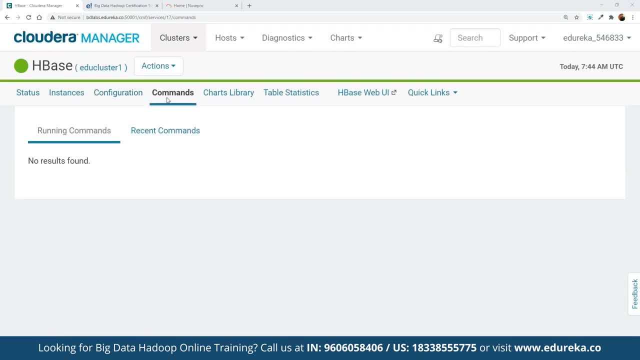 now to run some common commands. here we can simply see the list of all the commands that has been executed and in case they have been some recent commands executed on this one, then here we can simply see it. and here we can see the entire table statistics. if you want to work on the edge base ui, then here we can. 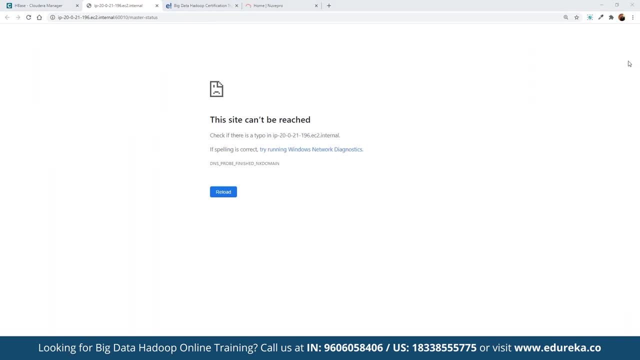 simply click on edge base web ui and then we'll be getting the access. in case we do have the access to this, so let's log into the console here so that we can start getting the access. just a moment, let's log into our console here, so here we can log in via the. 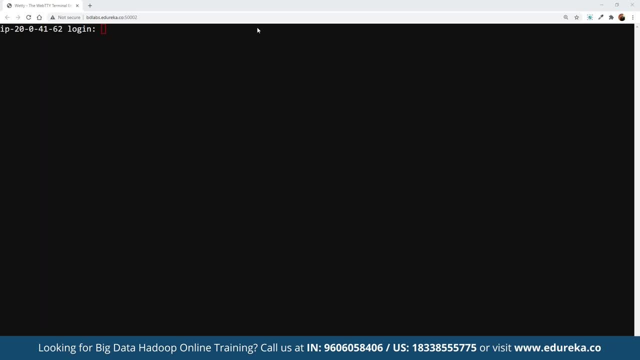 credentials here. let's do that just a moment. so here, once we have logged in again, we can simply type in different commands here as the edge base. now, for example, just to cross check if the edge base configuration has been properly defined or not, we can simply define the. 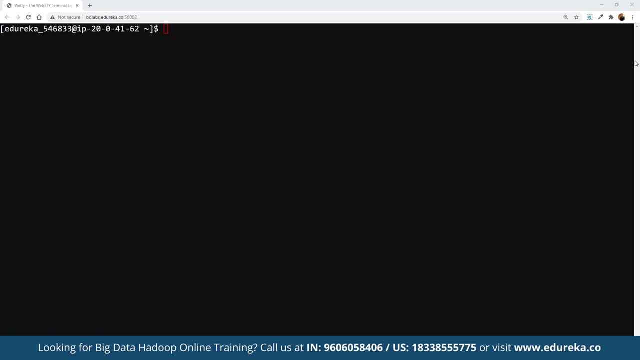 configuration for edge base and then we can write any commands once we have the access, so that we can get started accordingly now, in case we have now currently. this is what. this is basically the default console that we have if you want to work on the edge base shell. in case it has been. 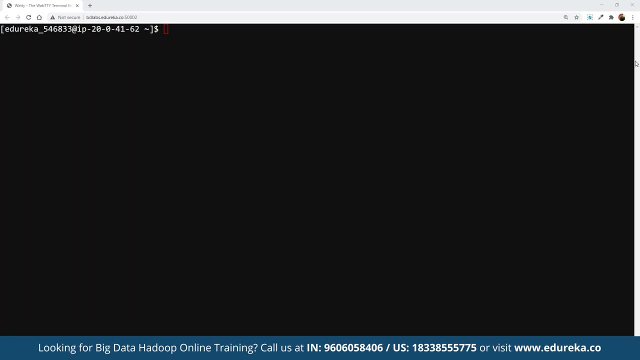 configured, then we can use the edge base shell and this, and then this is going to simply integrate the edge base shell. here and now we can simply get started. so whatever edge base tutorial code we want to work on, we can simply define the status. for example, to check the status for edge base. we. 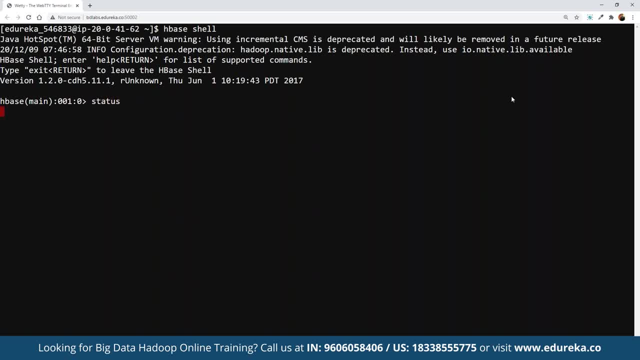 can simply use status and then status support for all the nodes up and running. so you can see, here we have one active master, zero backup masters, one server, zero dead and the average load here, so 763.67 is the average load and to see the current version of edge base being returned, we 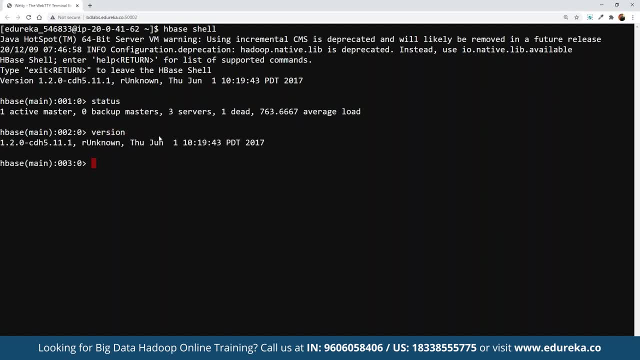 can use the concept as version, and then we can see that the current version has been 1.20, 5.111, and then we can see the timestamp as well, which has been done when it was properly installed, and then to see the list of all the commands for tables, and here we can define the. 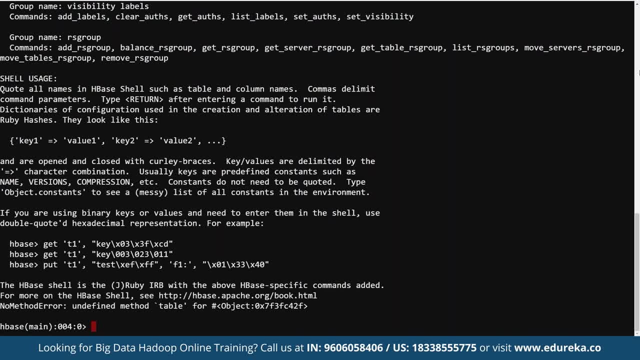 table and then here we can find health. so this is basically going to simply return all the help by a simple hyphen altogether. so here this is going to simply return all the statements which we can use along with table, along with the configurations defined here for edge base t1. 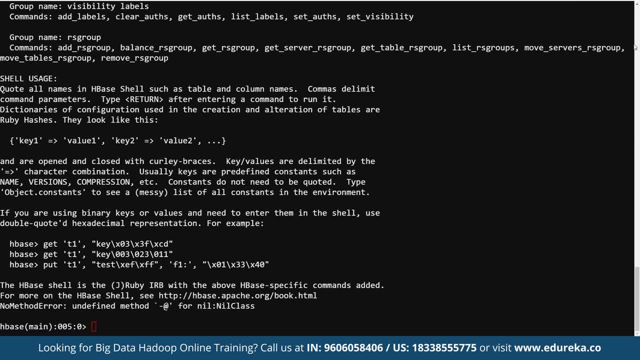 so now, for example, suppose, here we want to see the return, we want to see the result in terms of who's that we are, so here we can use who am i, and then we are going to see the user credential and you. This user is currently a part of this user group. 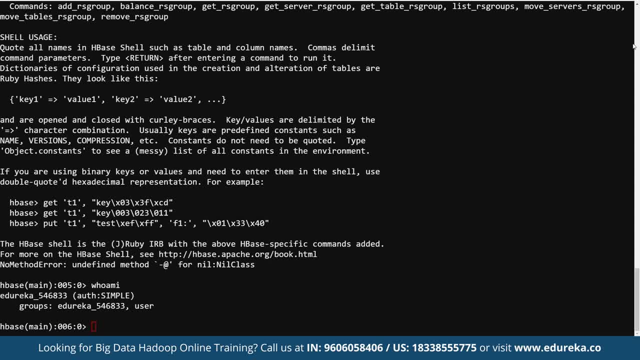 We can also see it as a result being specified here- And they are multiple again- If you want to work on the entire DDL part here. So, for example, suppose, if you want to create a simple employee table here, right, so we can do that. 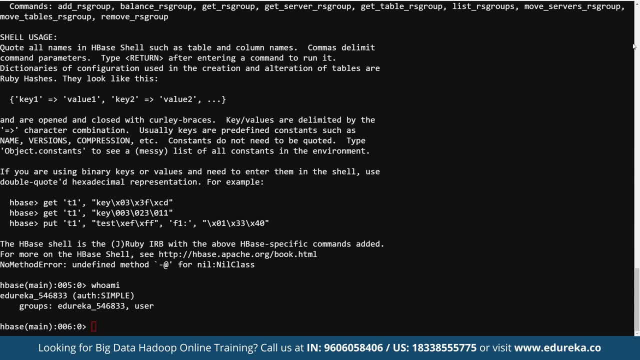 Since we are in HBase here, so we can define the entire. create table employee here. For example. suppose we are. our goal here is to create simple table for employees, So here we can define here. We can clear the screen now to create an employee table here. 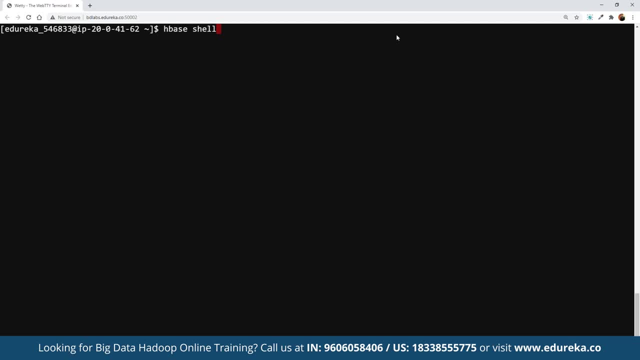 For example, suppose us to come out and then we can simply again reopen HBase shell. So here we can see the list of an offer to create a table here, For example. here we can define, create and suppose we want to create something for employees. 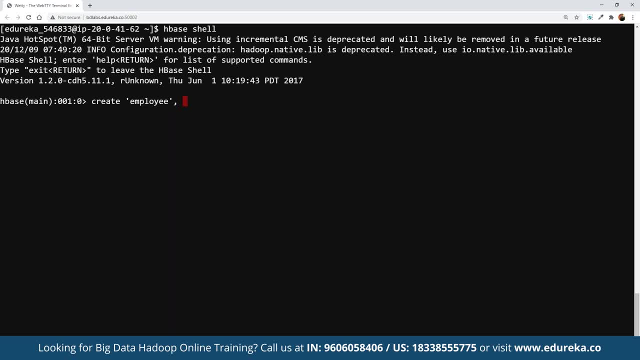 So here we can find employee, then we can define another column, suppose as name, and then we can define: suppose here We can define a simple ID column here. Now, here we can define ID, and let's say, here We've also want to add what we want to add something called 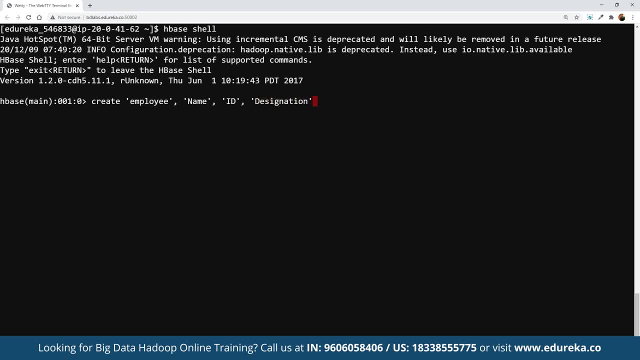 as designation, Then we want to add another column, suppose for salary or salary, and then we can add one for Department as well. So basically, here we are going to simply create one table for employees where we are going to define data set such as name ID, designation, salary and Department. 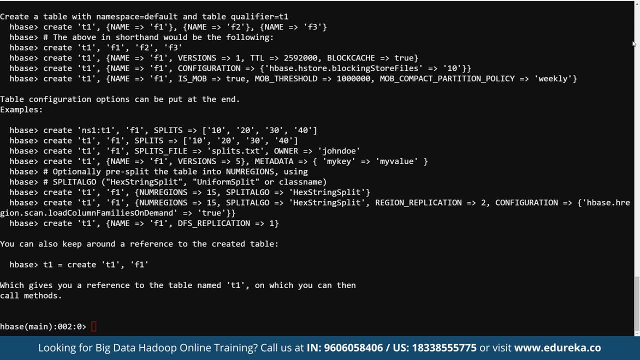 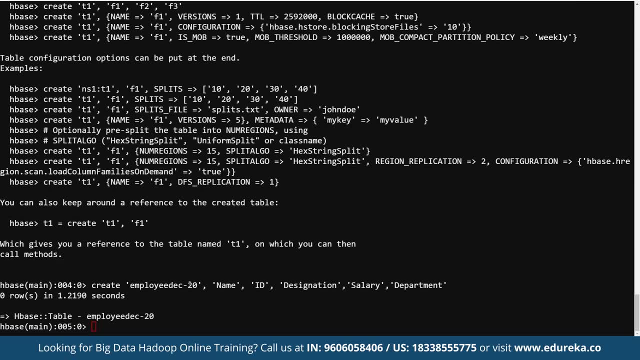 So if the table already exists here we can create a new table. Let's suppose here we can insert employee, here We can name it as employee one. So as you can see now we have changed the name here itself as employee December because again earlier the tables for 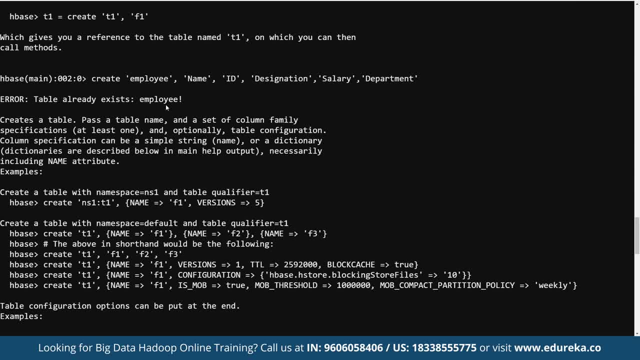 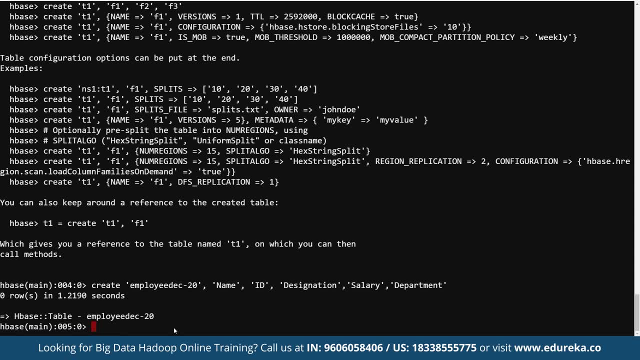 employee one, and employee has already been created in the past, So we cannot recreate that. So here we define a new name And now, if you want to start working on one specific table, so here we can define table and then we can define which table. 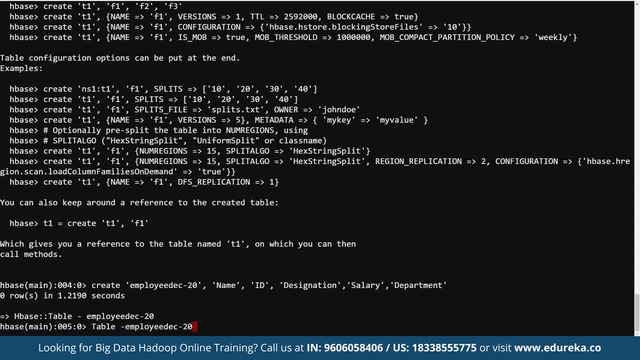 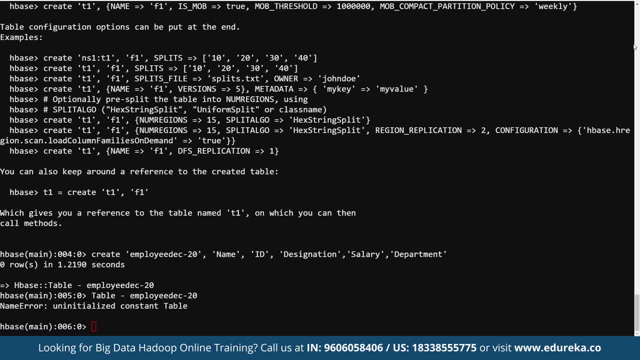 you want to work on, suppose, employee December 20, that we have defined just now. So here we can find the table name as well. Whatever we have defined, You know, since we have switched to that table, here we can see the table name is also being returned to us. 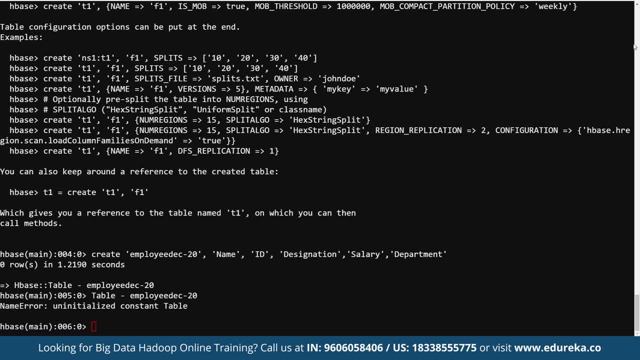 That means now we can start working on this particular table itself. right, And now suppose Let's say here we go back to the same cloud data manager, We will be able to see our new region will also be created for the table that we have defined just now. 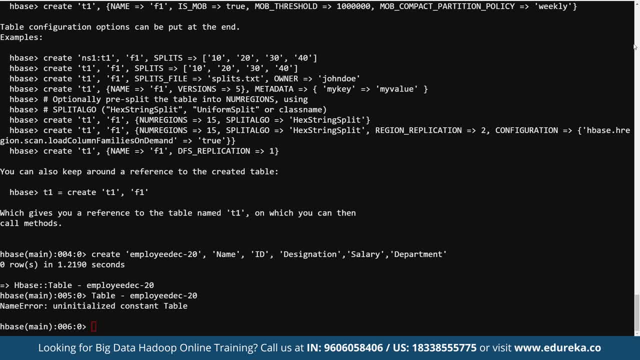 All right. So now, if you want to see the entire list of all the tables here, then here we can use command as list and you can see that currently there are multiple tables being created here, So we can see the list of all the tables being returned to. 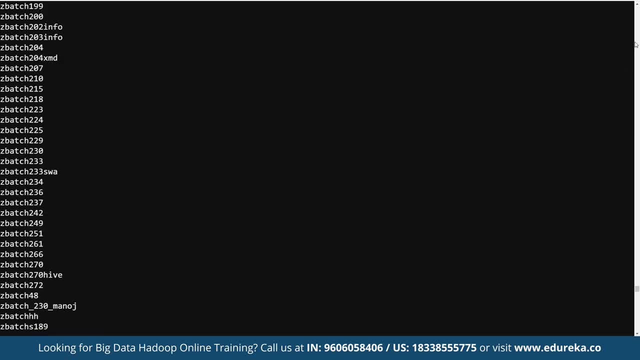 us. and same way, if you go back now to see the details in our edge based dashboard, We can go back, and in our edge based dashboard here we have to go to a simple region dashboard here. So let me show you how exactly we can go ahead. and so here we. 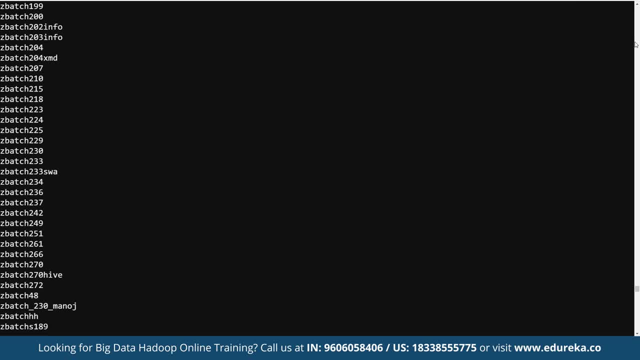 can see the status here, and then for the edge base, we can see the region. here We can see the report for every region that is currently available here and now. to see the report for which all regions have been created, We can go to the section for status. 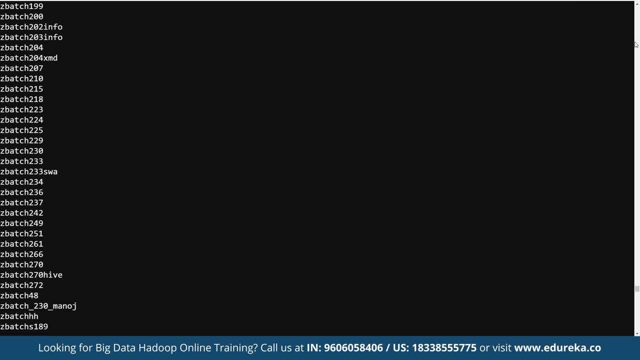 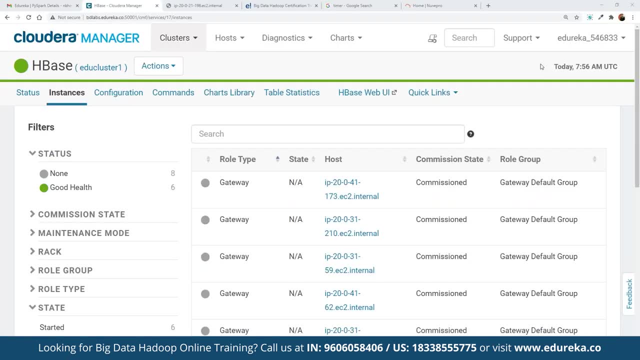 And then we will be able to see the region in which it has been applied so that we can have a quick insight on it. So that's how we can get started working on any edge based environment. as for the set of required, and same way if you. 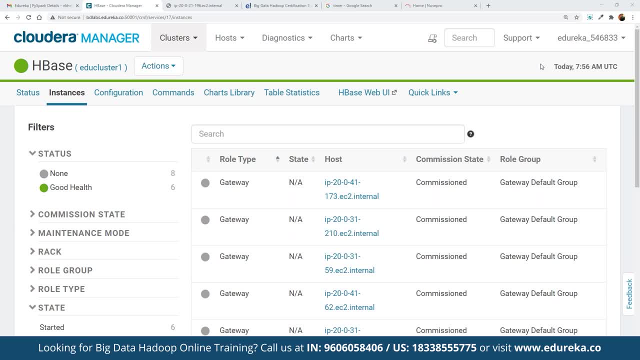 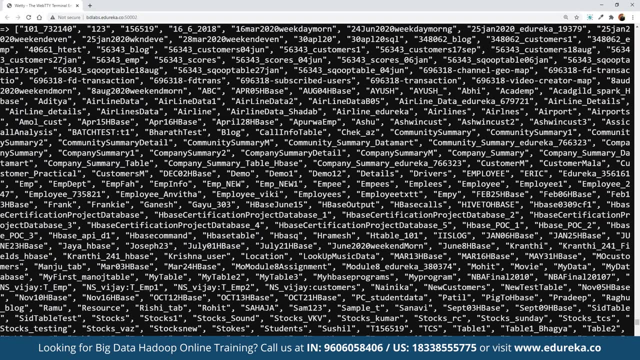 want to work on creation of more tables here, because, again, at the end, this is what a simple, no SQL structure is and suppose we want to work on the SQL structure. we can simply get down and can. So these are the list of all the tables currently available. 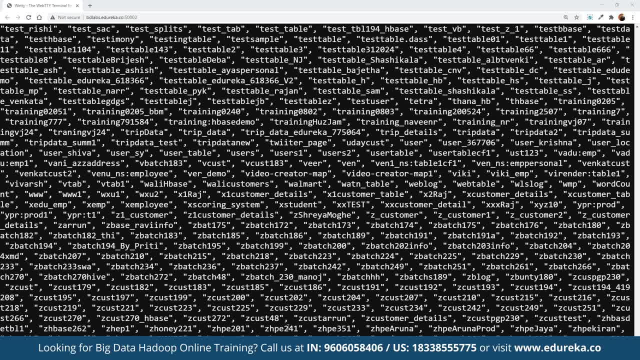 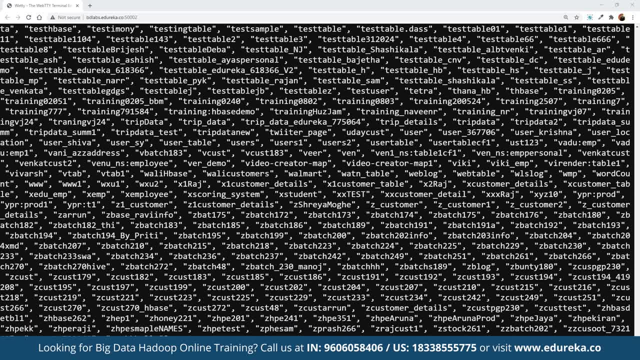 here Now, for example, suppose I say for any reason, suppose we want to disable the current table that we had, we did here's I, so here we can simply happen as disabled. I think has frozen, So let's refresh the connection just a moment. 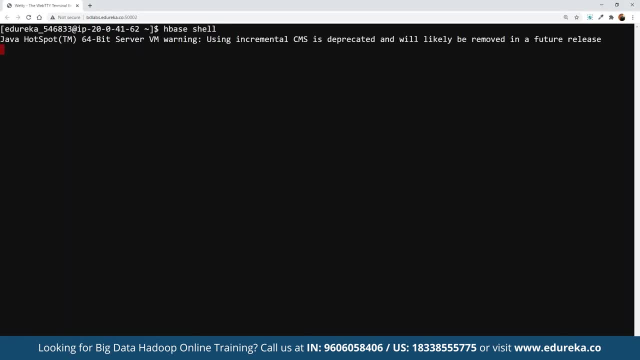 We can again restart HBase, HBase shell, as opposed to say here, once we have moved into that HBase shell. suppose now and suppose here we want to disable one particular table, So here we can use disable, And then suppose here we want to disable December employee. 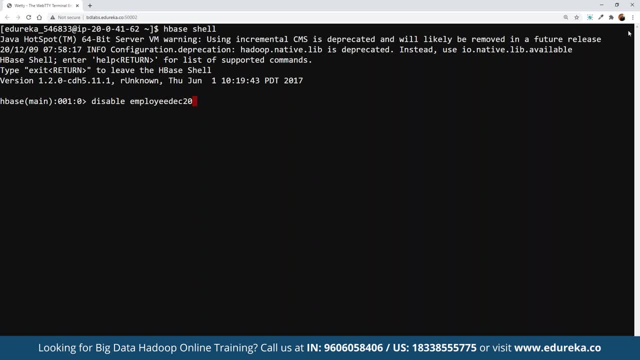 December 20 that we have created. So here we can define a table name. and if you want to disable the store here- we don't want to use this as a part of region right now- then we can simply do that. Suppose here we want to work on one specific table, then we 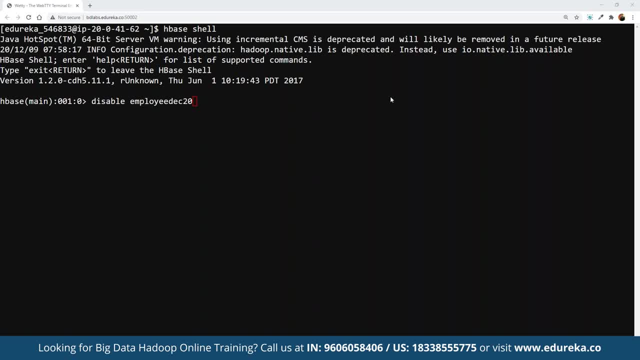 can define the table and the name for it. suppose here we have employee December 20. Then we can see the entire report also being generated here. So we are going to work, work on more references as you put, as you proceed further. So let's say, here we want to create another scripture. 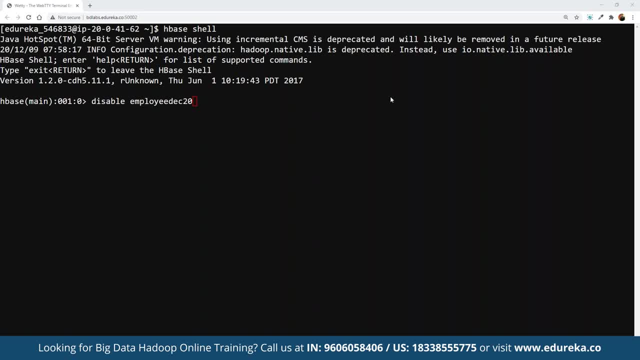 For example, let's say: here we can come out and let's say we clear the screen here. Now we want to work on some other scripts. If was, I will here we define: Okay, how we can create a table here, how we can display disable. 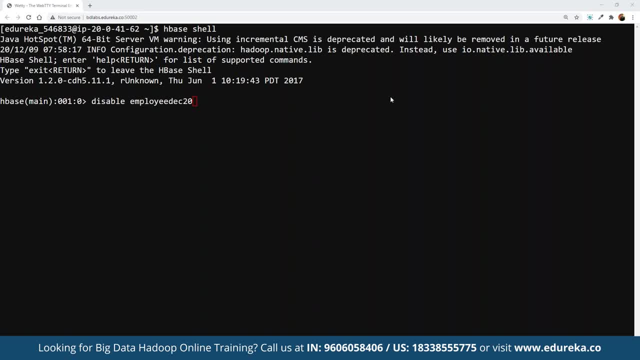 multiple tables. now, for disabling multiple tables, We are going to be simply use the small statement. now We can disable a single table that we had done, or we can use multiple tables for for again, If you have requirement of the sleeping wonderful table, such ones, and we can simply use a statement as well as in required. 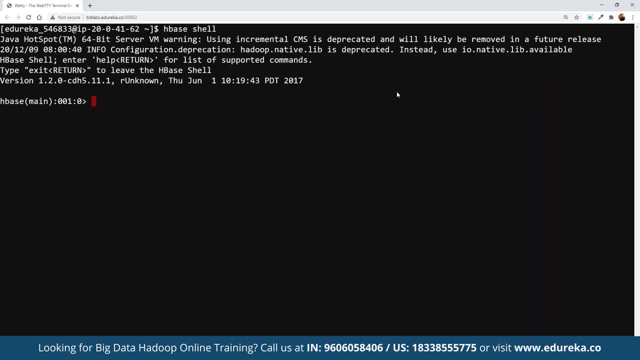 So the create table was what we had seen before. So let's suppose we do one thing, Let's create another table as create, and then we can disable all the tables here. So here we can define suppose as employee or employee, and that will for December. 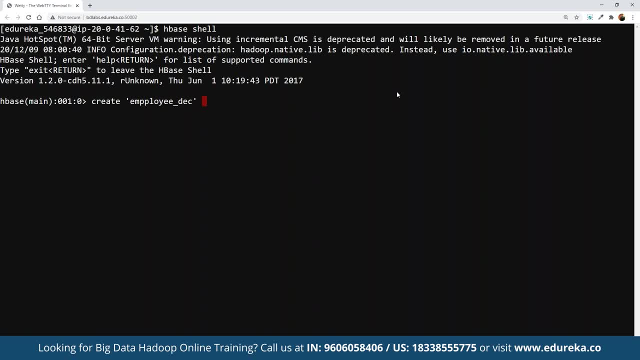 As a name and name. We want to create another table having, suppose, its own name. Then we may have value for ID, Then we may have value for designation. Same way, here We are going to have value, suppose again, for salary, And one more. 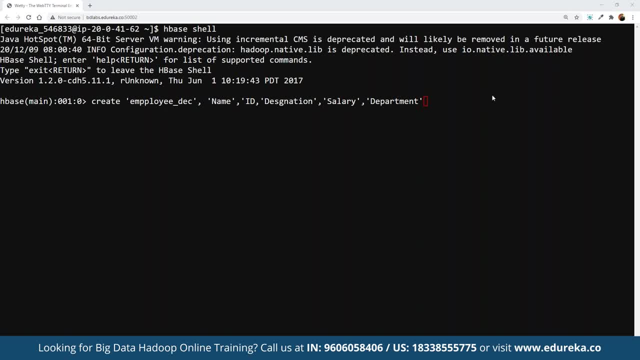 For the department. So here we can define this table by this name here, and then we will be able to work on this specific table itself. So here we can disable now if you want to disable all. so here we can define, define statement as disable all, and then if you 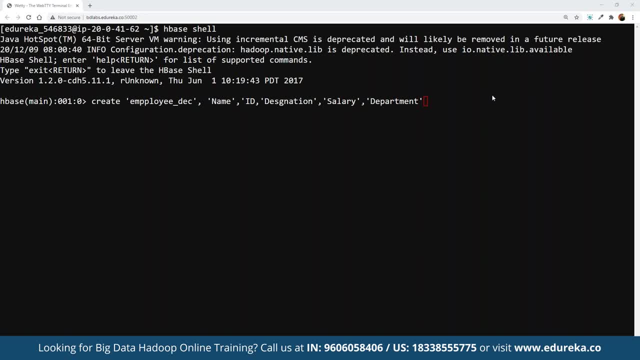 want to disable all the tables having the prefix as e and any specific table structure that we can define the parameters. Yeah, so this is going to find out. all the tables starting from here and again can continue to any of the elements that you want to define hands. 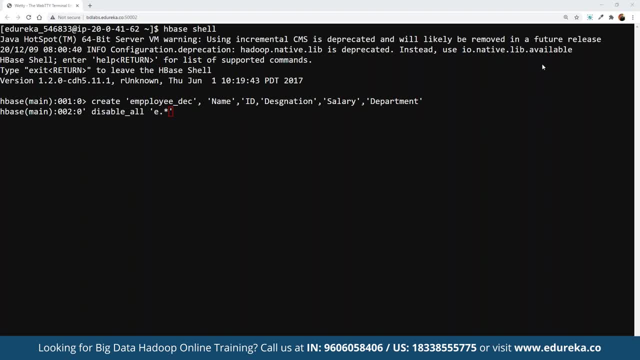 For example, if they are multiple tables by the e, then they all are going to be disabled for now, as opposed, if you want to see the list of all tables having this structure, that we can simply press enter and then we will be asked a simple confirmation. 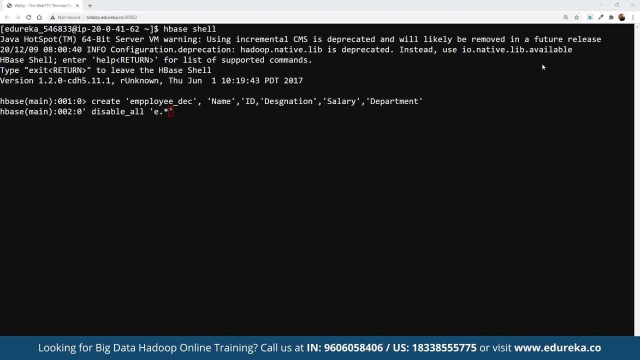 if, yes, we want to disable all the two tables or not, and in case there are no two are no tables created as of now, then this is going to be simply done as a Blank value And if you are looking to put any, I can say: add any entries. 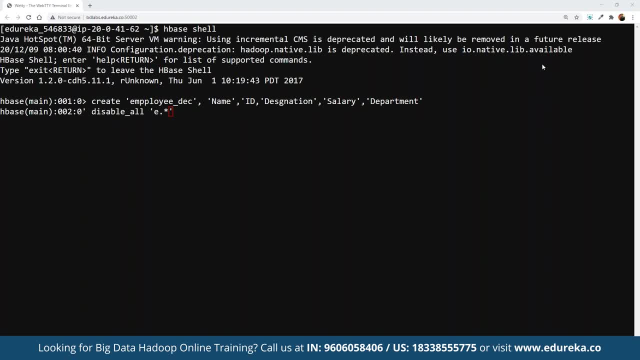 to any of the table. For example, we had a fine table as employee December right. So now we want to put any entries here. So here we can use a command as put and then we won't have to define: Okay, we win, which table we want to put the put the details. 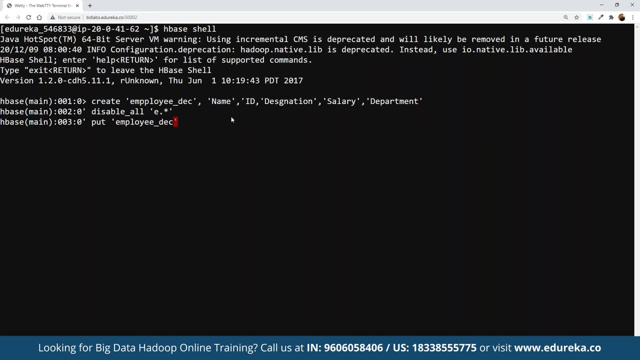 Here We have employee for December. now in this table We are going to define the. we have to find the values As well. For example, your name is suppose John, So here we can define the name as John, and then we can here. 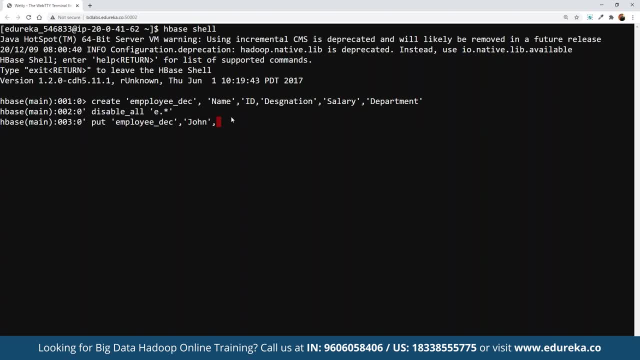 we have what? here we have name. so you can keep on defining multiple tables, multiple values as part of the requirement. here We can define any values as part of the requirement. So, for example, suppose here we want to define any specific value of example name, full name, or we want to insert any values. 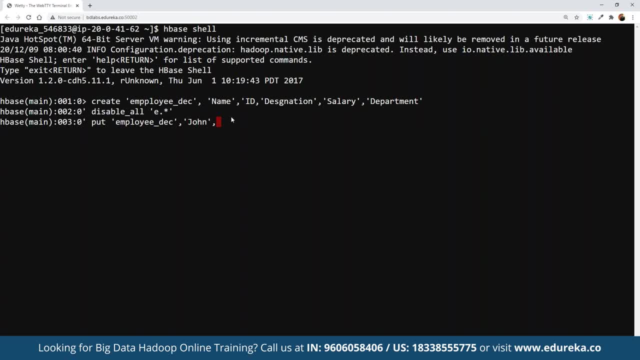 as a part of the newest database. So we can. We can also define that. for example, here we can define the name. next we can define, suppose, the name as name, as a full name. So here we can define full name. and suppose, here we can define: 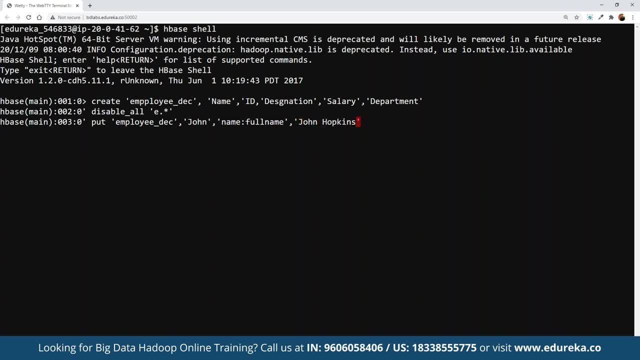 full name, as it was John Hopkins. So again, you know it can be any name and if you run this on this current table that has been created, we will be able to see the entry is going to be updated here. So that's how we can start. 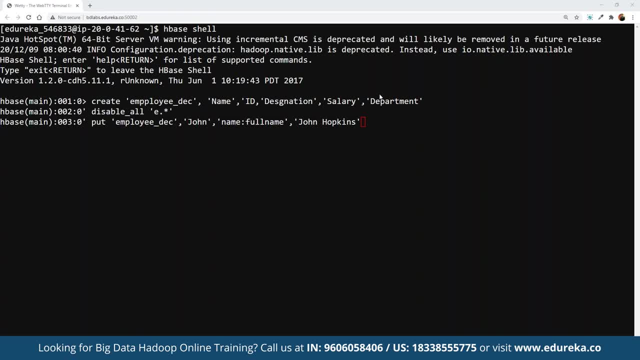 I'm manipulating it. And again, if you want to add more details here, we can define this for a suppose, same way We also want to import, or can we also want to insert the details for age as well? So here we can keep the name as same and then we have, we can. 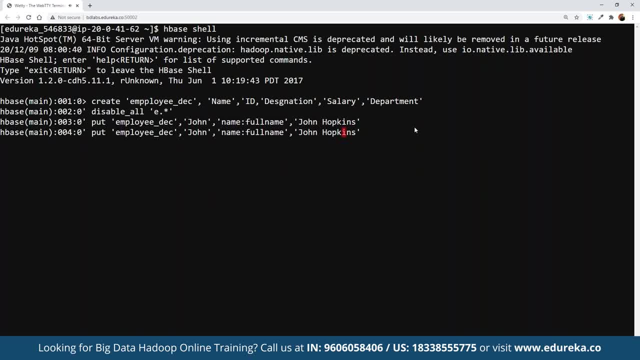 find the present. if, example: here we can define present age instead of full name We can give, we can go for present age, Suppose age as a present age, and here we can define the by suppose a present age is for present Age, as opposed. 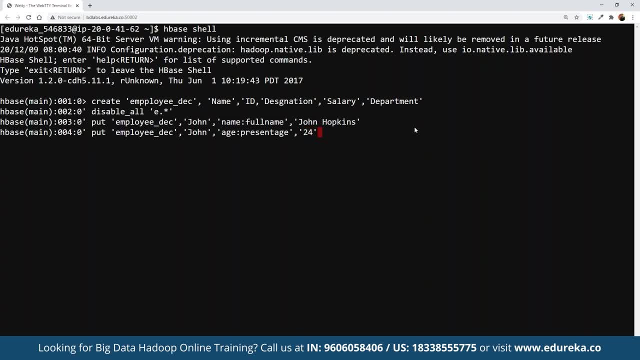 Let's say 24, if we can find present age, and then we can define the course or we can say any name that you want to be referred. So that's how we can keep on and on adding entries here. Thank you so much for joining guys and have a great day. 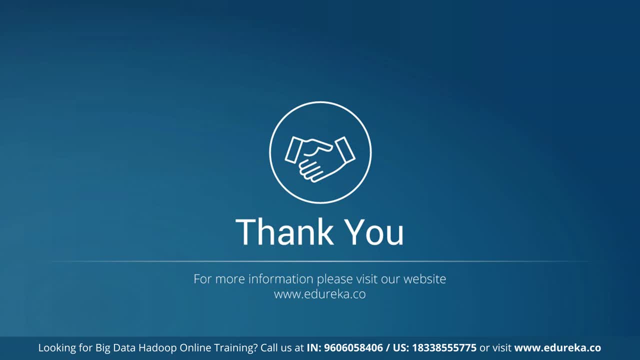 Take care. Bye, Bye, Bye, Bye, Bye, Bye.